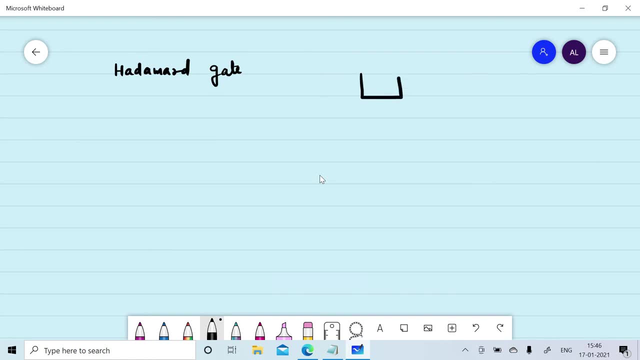 Hadamard gate can be represented by H. It will consider a single qubit as input and it will generate a single qubit in output state. It is represented by matrix 1, by square root of 2, 1, 1, 1 minus 1.. Consider we have a qubit in zero state and we apply Hadamard. 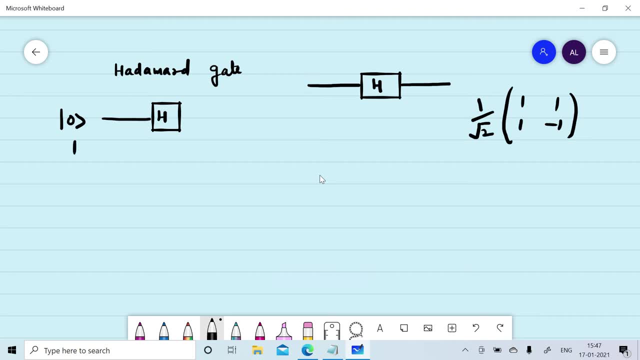 gate. So zero state can be represented by matrix 1: 0.. So what we will get is 1 by square root of 2, 1, 1, 1 minus 1, and qubit 0 is represented by 1: 0.. So 1: 0, we will get 1 by square root. 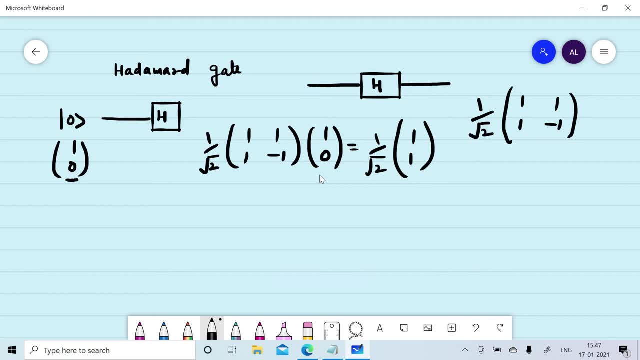 of 2, 1, 1, which can be represented by 1 by square root of 2, qubit in zero state, plus 1 by square root of 2 qubit in one state. So if we will consider a qubit in zero state as input and we will apply Hadamard gate, 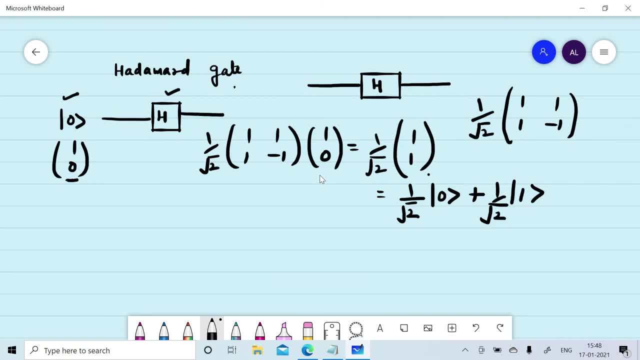 we will get the qubit in superposition state, that is, 1 by square root of 2 in zero state plus 1 by square root of 2 in one state. Similarly, if our input qubit is in one state and if we will apply Hadamard gate, 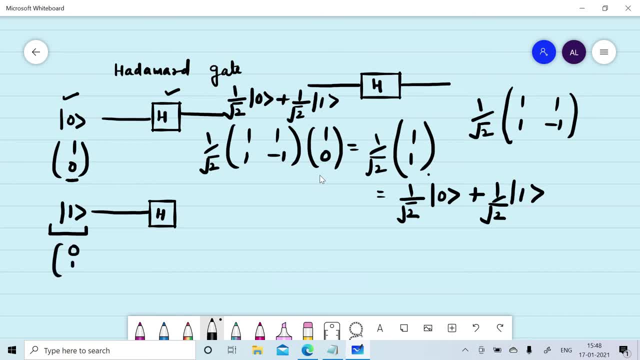 the qubit in one state can be represented by matrix 0, 1.. On applying Hadamard gate, what we will get is 1 by square root of 2, 1. 1, 1 minus 1, 0, 1.. 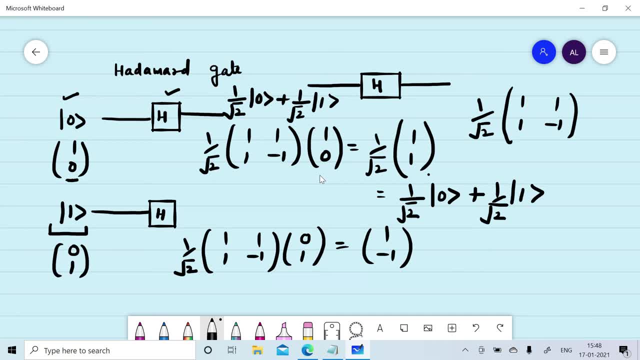 So we will get 1 minus 1 and 1 by square root of 2.. It can be represented by 1 by square root of 2 in zero state, minus 1 by square root of 2 in one state. On applying Hadamard gate. 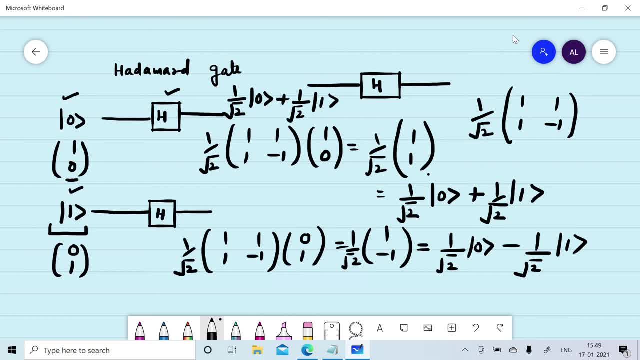 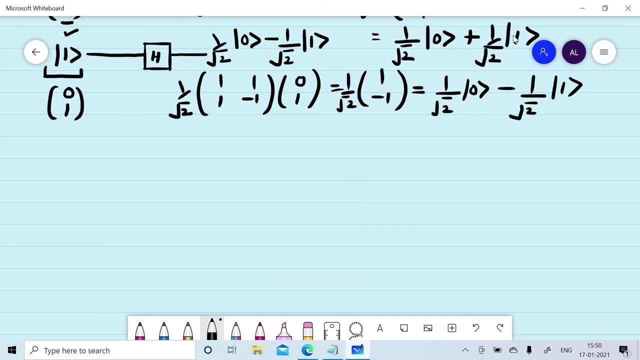 to a qubit in one state, we will get a superposition state 1 by square root of 2 qubit in zero state minus 1 by square root of 2 qubit in one state. Now we will consider the case where the input qubit is already in superposition, that is, 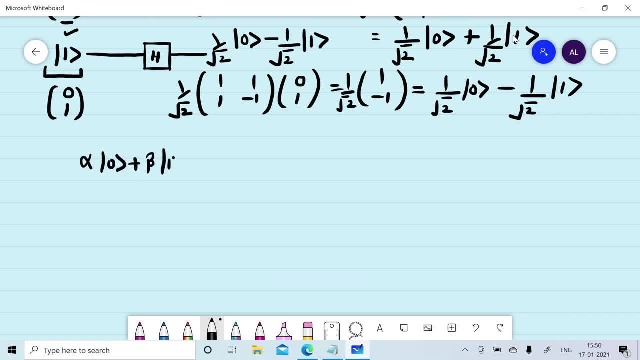 alpha 0 plus beta 1 and we will apply a Hadamard gate. Input qubit is represented by a matrix alpha beta. On applying Hadamard gate, we will get a superposition state 1 by square root of 2 in one state. 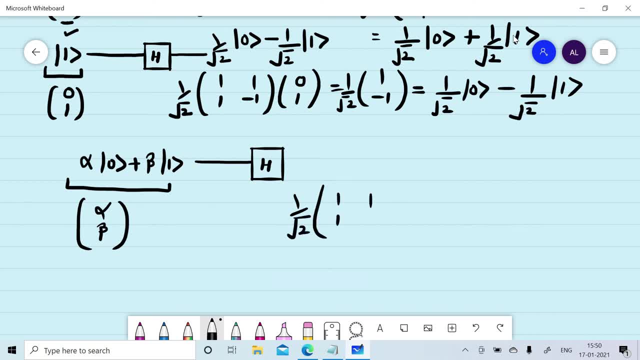 And on applying Hadamard gate, we will get 1, 1,, 1 minus 1, qubit is represented by matrix notation. alpha beta: We will get 1 by square root of 2. alpha plus beta, alpha minus beta, which can be further. 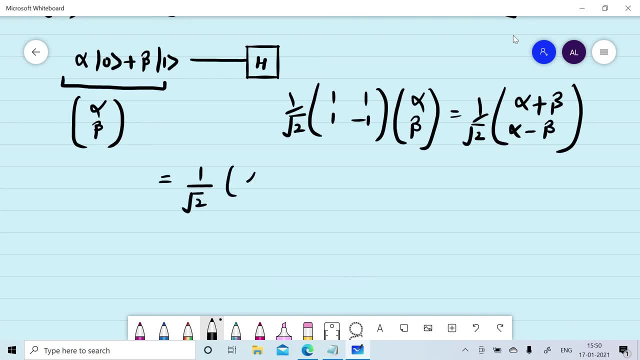 represented by 1 by square root of 2 alpha plus beta in zero state, 1 by square root of 2 alpha minus beta qubit in one state, Which can be further represented by 1 by square root of 2 alpha- 0 state plus 1 state plus 1 by square root of 2 beta qubit in 0 state minus qubit in 1 state. 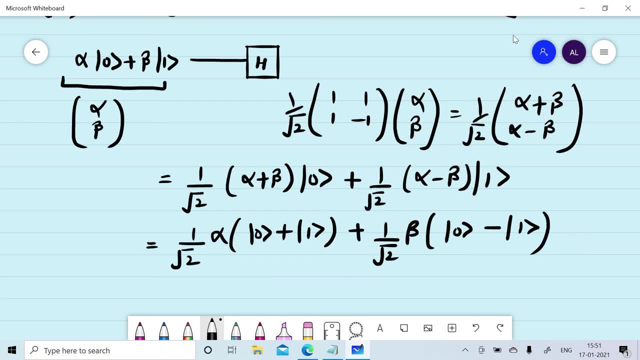 So, on applying Hadamard gate to a superposition state, we will get 1 by square root of 2 alpha 0 plus 1 plus 1 by square root of 2 beta qubit in 0 state minus qubit in 1 state. 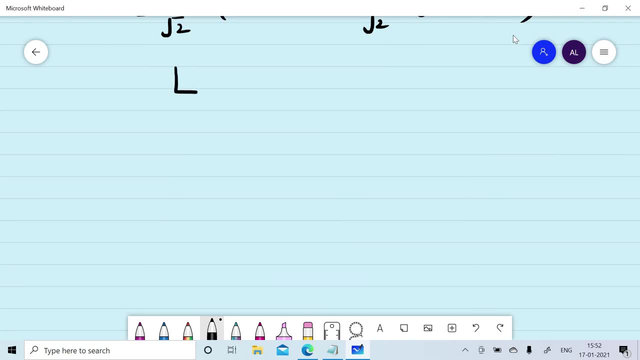 Hadamard gate is reversible in nature. It means if we will apply Hadamard gate twice to a qubit state, we will get the original state As the outcome, like if we have a qubit in 0 state. we will get the qubit in 0 state after applying Hadamard gate twice. 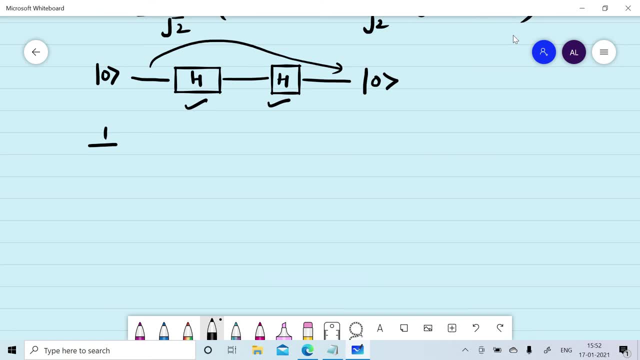 So let's verify it. Hadamard gate can be represented by 1 by square root of 2, 1, 1, 1 minus 1.. Qubit 0 is represented by 1, 0.. So at this point of time, we will get 1 by square root of 2, 1, 1.. 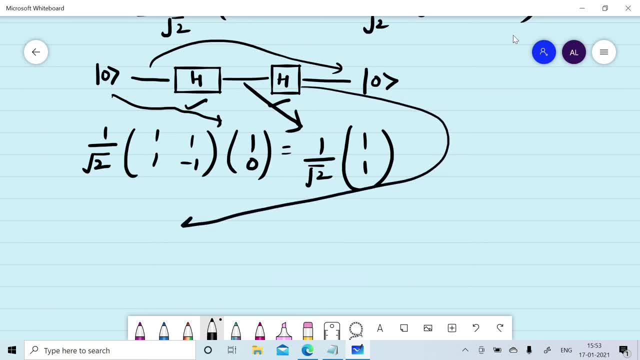 Then we will again apply the Hadamard gate. So Hadamard matrix is represented by 1 by square root of 2, 1, 1, 1 minus 1.. Our qubit is represented by 1 by square root of 2, 1, 1.. 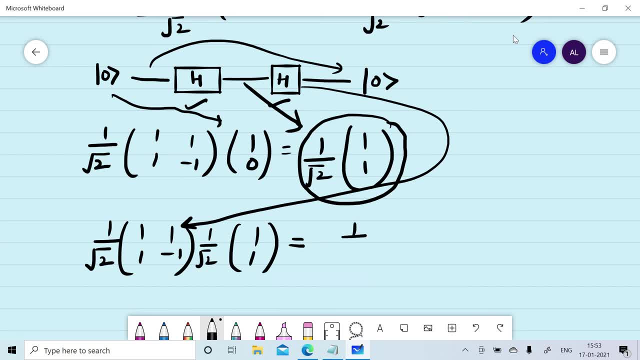 If we will apply the matrix multiplication, we will get 1 by 2, 2, 0, which can be further represented by 1, 0. That is nothing but a qubit in 0 state. Similarly, if we will apply Hadamard gate twice to a qubit state, we will get 1 by square root of 2, 1, 1 minus 1.. Similarly, if we will apply Hadamard gate twice to a qubit state, we will get 1 by square root of 2, 1, 1 minus 1.. Similarly, if we will apply Hadamard gate twice to a qubit state, we will get 1 by square root of 2, 1, 1 minus 1.. 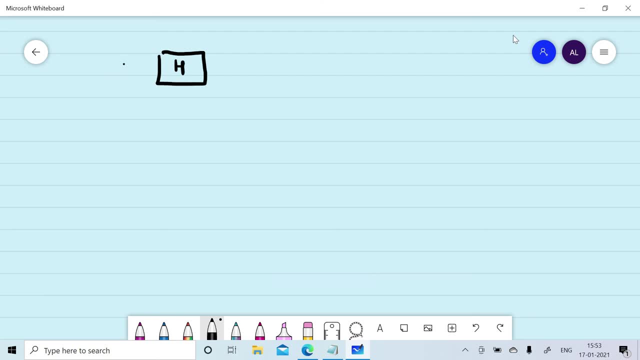 Secondly, if we will apply Hadamard gate to a qubit in 1 state and second time we will again apply the Hadamard gate, we will get the output as qubit in 1 state. Let's verify it: 1 by square root of 2, Hadamard gate is represented by 1, 1, 1, minus 1.. 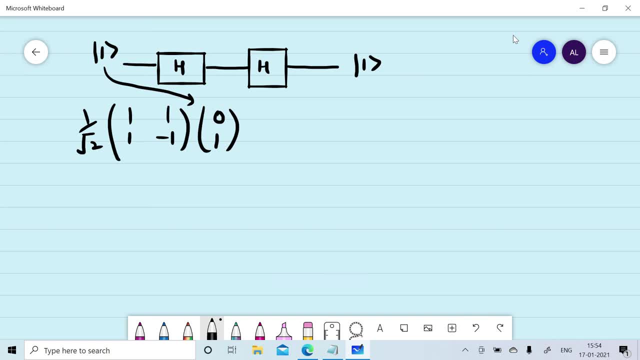 Qubit in 1 state is represented by 0, 1.. So we will get 1 by square root of 2, 1, minus 1.. Again, we will apply the second Hadamard gate, that is, 1 by square root of 2, 1, 1, 1, minus 1.. 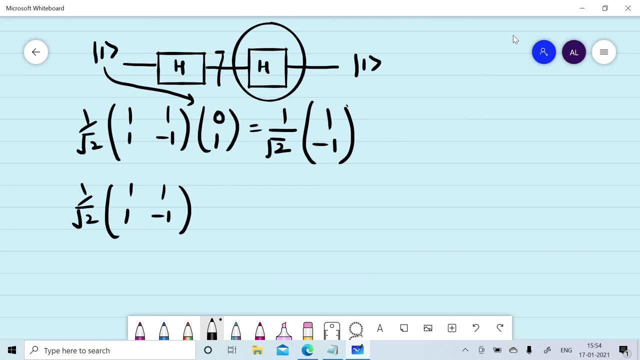 And the qubit at this point of time is represented by matrix 1, by square root of 2, 1, minus 1.. So we will get 1 by 2, 0, 2, which can be further represented by 0, 1.. 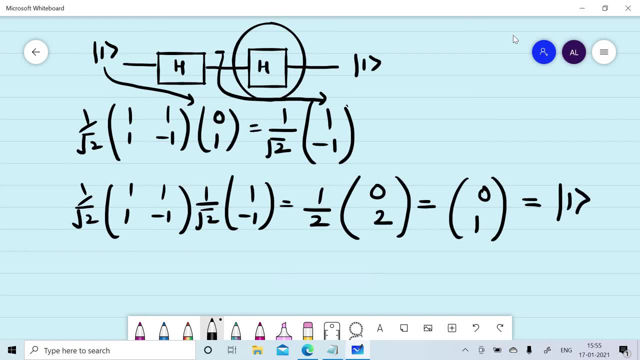 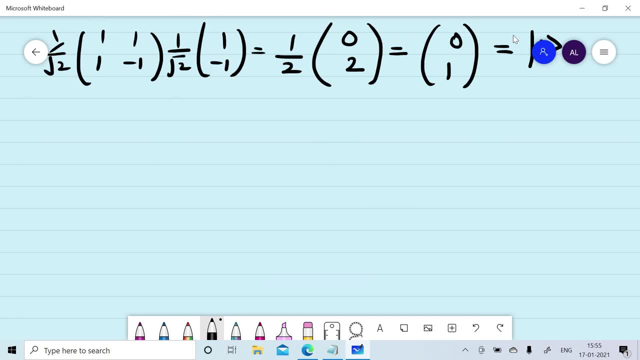 And that is nothing, a qubit in one state. So in summary, we can say a Hadamard gate is reversible in nature. You can verify the same for a superposition state and apply the Hadamard gate twice and observe whether you will get the same superposition as the output or not. 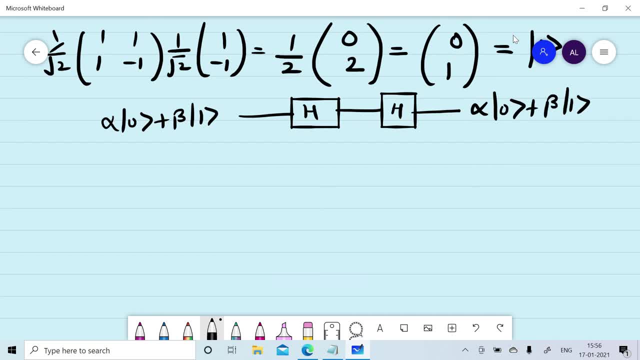 So in summary, we can say: whenever we will apply a Hadamard gate to a qubit in 0 state, we will get 1 by square root of 2, qubit in 0 state. So in summary, we can say: whenever we will apply a Hadamard gate to a qubit in 0 state, we will get 1 by square root of 2, qubit in 0 state. 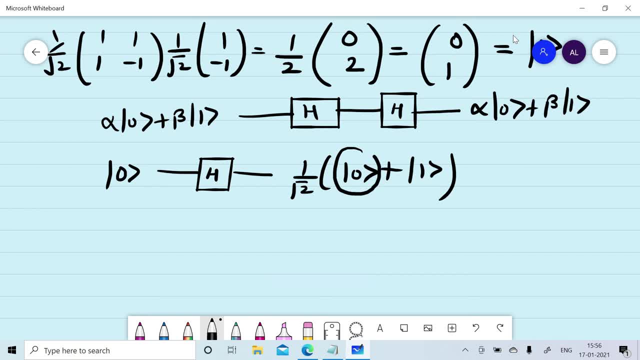 It means that, if you will measure it, there is 1 by square root of 2,- that is, 1 by 2- probability that we are in 0 state, And 1 by square root of 2,- that is 1 by 2- probability that our qubit is in 1 state. 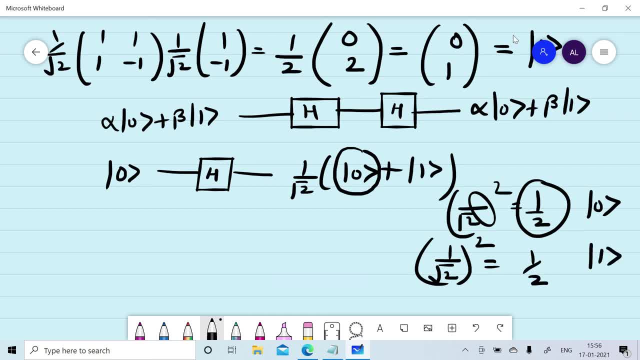 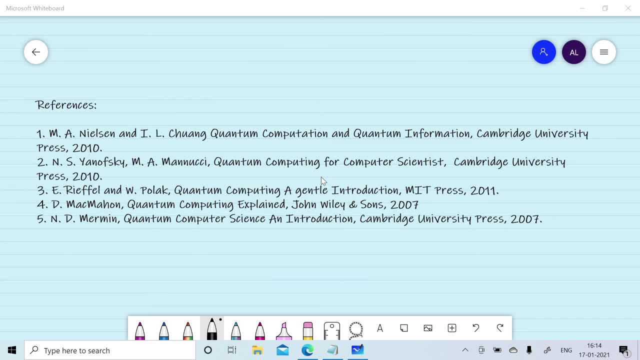 So in this session we had discussed the concept of Hadamard gate and apply Hadamard gate, create the superposition state. These are the references. Thanks for watching this session.